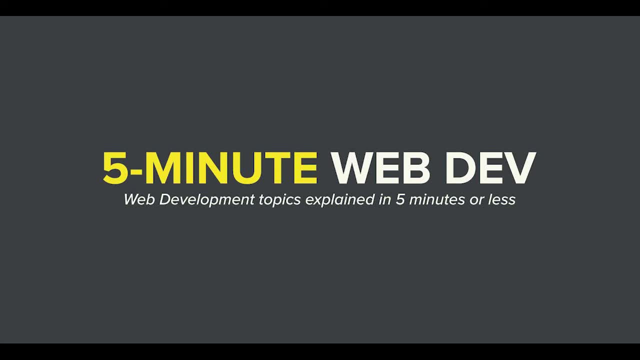 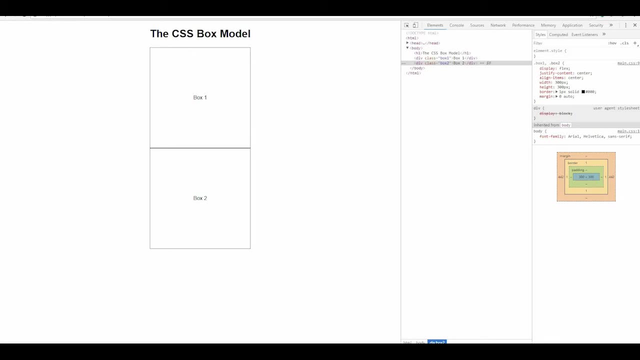 Hey everybody, you're watching 5-Minute Web Dev and today we're going to learn some CSS. Hey everybody, my name is Zach and I want to thank you for joining me for the very first episode of 5-Minute CSS, where I explain CSS topics that you want to learn about in 5 minutes. 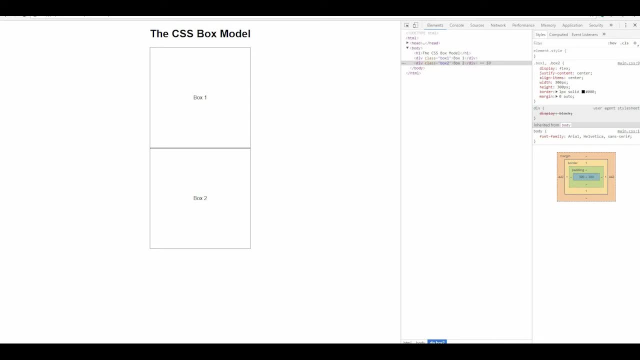 or less. Today's topic is the box model. The box model is probably the most important and foundational concept to understand when you begin working with CSS and styling webpages. Each element on a webpage is a box. Each box has four different areas: content, padding. 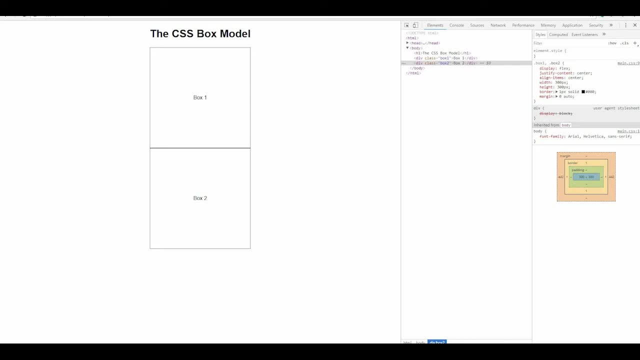 border and margin. We're going to go through each of these and in 5 minutes you should have a solid understanding of the box model. Now, really quick, I want you to picture a property in your head, Not a CSS property, but an actual property: A house, a lawn, a fence, And as we 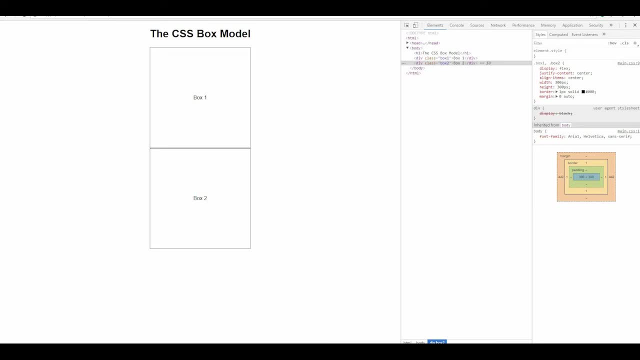 move forward. I want you to keep that picture in your mind because I think it's going to really help you a lot. Alright, let's jump right in. First up, the content area. The content area is where the content of your element lives, So your text nested elements, things like that. 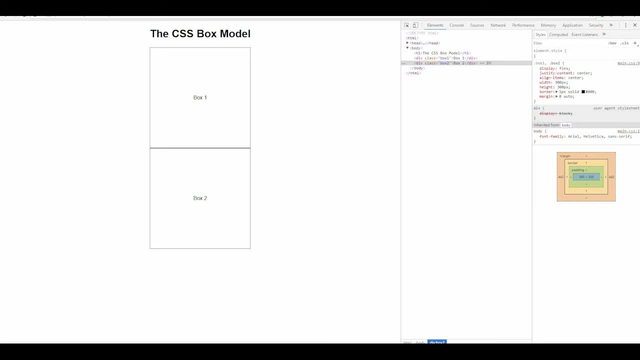 they all live within the content area. Using our analogy, the content area is the house. Width and height properties are applied to the content area by default. Now there's a way to change the way that works, but we'll go over that in another video. on the box sizing property, When we talk about it. now we're going to talk. 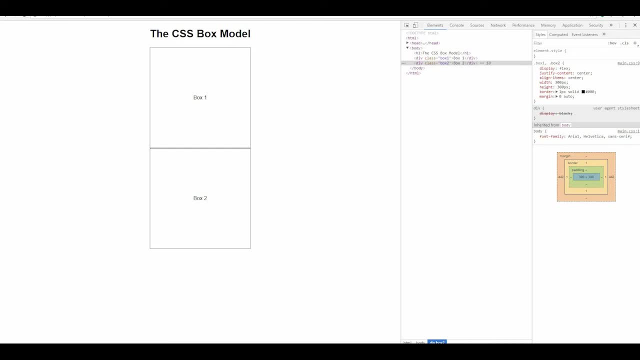 about it in the default context if you were to start writing CSS. okay, So when you say a width of 300,, like I have, and a height of 300,, it gets applied to the content area, which you can see pictured in blue here. Let's ignore the extra two pixels and the black which is the border. 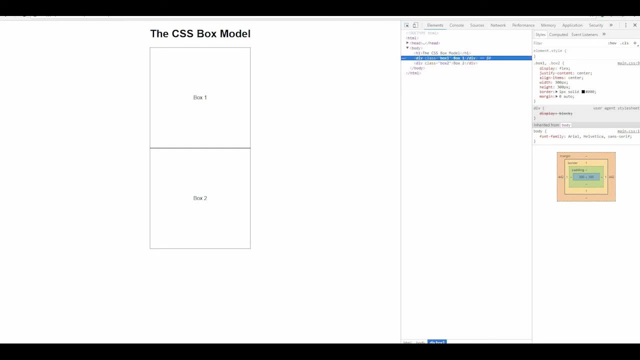 we'll get to that in just a few minutes, okay, Moving on, we have padding. Padding is the space within an element. It's a space between the content of the element and the border of the element. In our analogy, it's the lawn or it's the area around the house, between the actual building and. 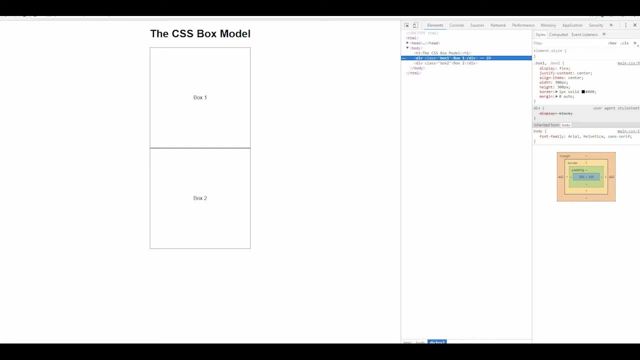 the fence. The values for padding are set with the padding property. These values increase the total width and height of our element in addition to the width and height set on the content area. So if I go ahead and add a padding of 20 pixels to our boxes here, 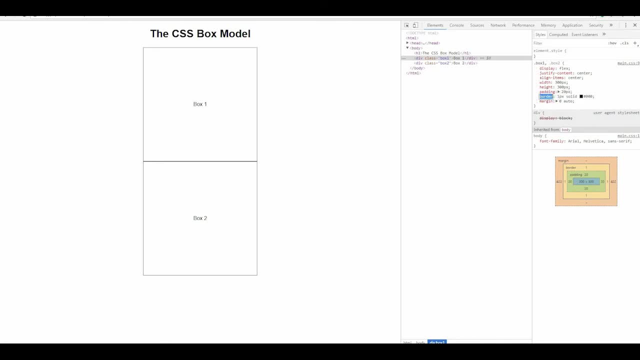 that's going to add 20 pixels on each side, top right, bottom left- for a total of 40 additional pixels of width, 40 additional pixels of height. You're going to see we now have instead of 302, or. 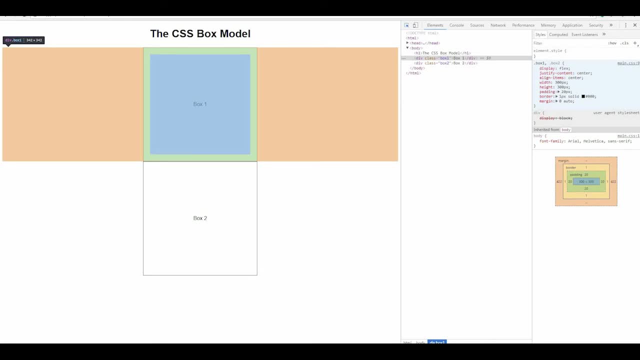 300, which we had. we have 342 by 342, and it's pictured in green there. So that's padding. If you want to make space within your element or allow your element room to breathe in relation to itself, in relation to its content, use padding. Moving on, we have the border, The 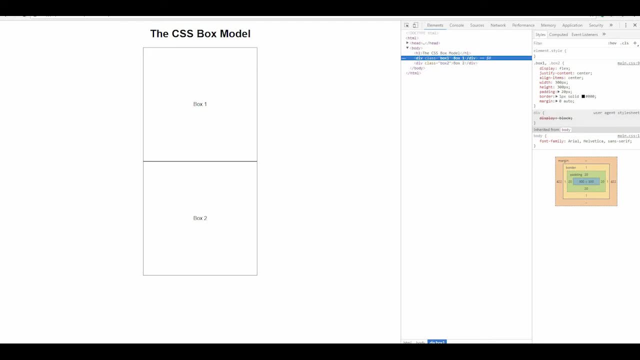 border is the space between the content area and the border of the element. So if I go ahead and add a border, I can see that the border is the fence in our analogy. I think it's simple enough to reason about. In the real world, it's the fence that separates us from the rest of the world. 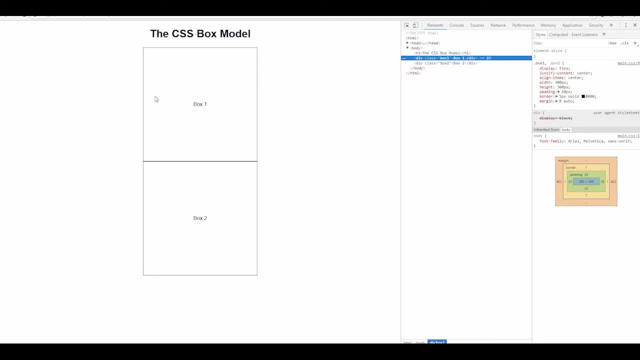 but it still adds to the size of our property. in a sense, In CSS, the border, its width, still adds to the width of the total element and it's what separates us from the rest of the web page, basically. So if you have our border, here, I have a border of one pixel. 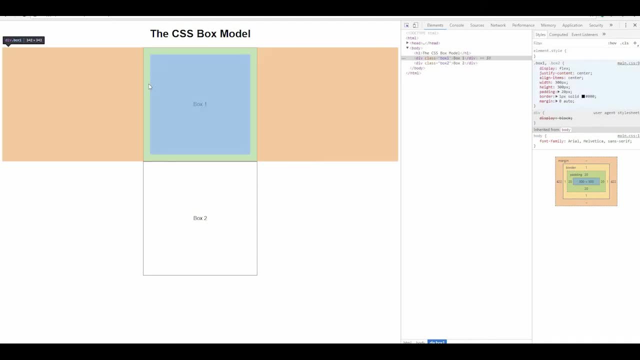 so one pixel on each side is two pixels and that's where we get that extra two pixels. That's why it's calculated there 342 by 342.. We can see it in black here. That's border. Moving on, we have the margin. The margin is the space between your element. 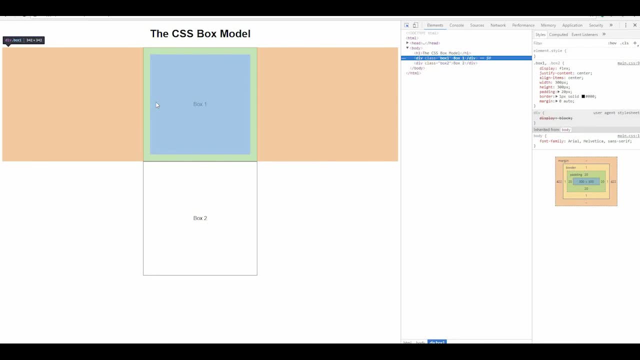 and other elements. Right now, I want you to ignore the margin on the left and the right. I'm going to go ahead and add a margin bottom here. That's 20 pixels. You're going to see it just created 20 pixels of space between box one and box two. I added that margin just to box one. 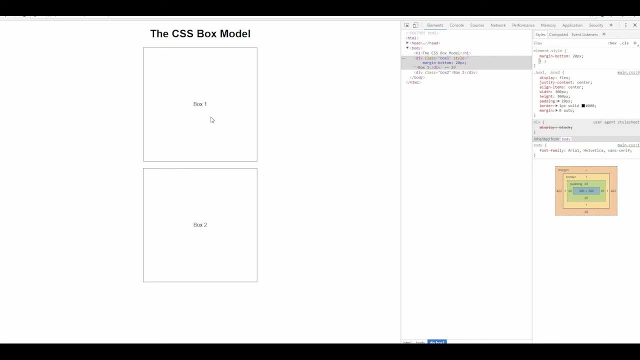 The margin is still technically defined within the context of the specific element, but it is not included in the size of the element. That 20 pixels didn't get added on to the 342.. The total element size is still 342 by 342, but really it's just a different.